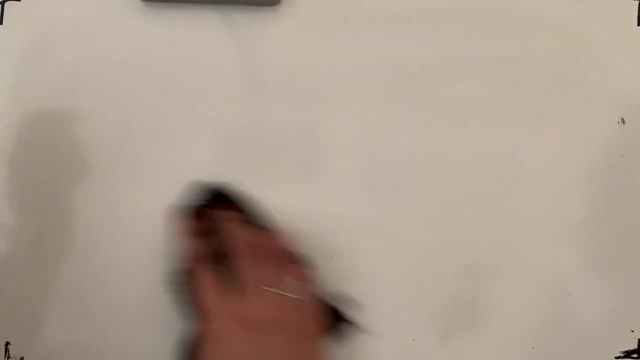 And two key words I just want to discuss are a parent compound and a substituent Right. So the parent compound, for example, if we just go for this compound over here, OK, the parent compound in this case is the longest carbon chain. 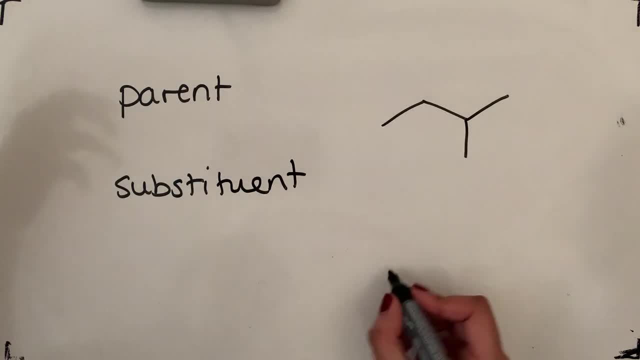 And in this case it is a butane chain. The parent name always goes at the end, So this name is going to end in butane. The substituent is any branches or other atoms coming off of it, And in this case we've got that methyl coming off of that parent butane chain. 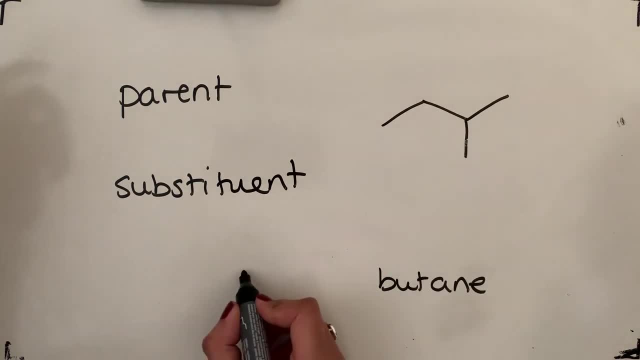 It's coming off of the second compound And therefore the substituent is called 2-methyl And the substituent name goes at the beginning, The parent name goes at the end, So this molecule over here is called 2-methylbutane. 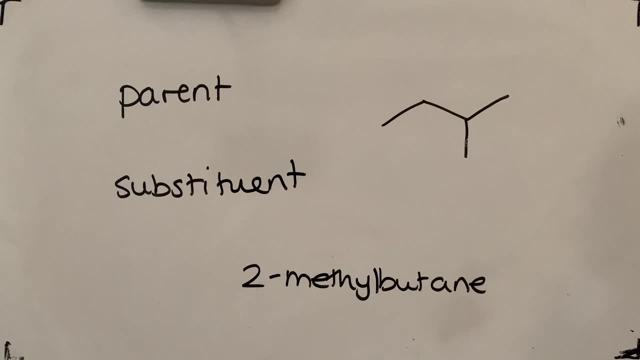 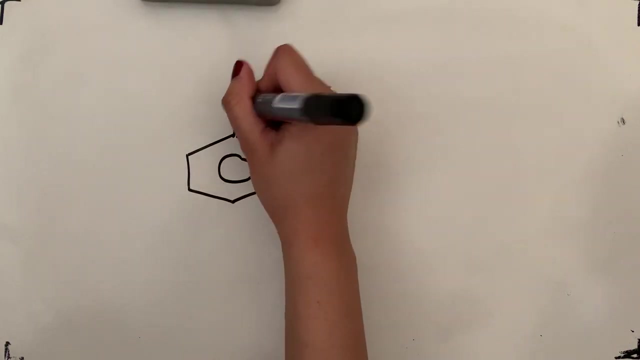 We're now going to apply the same principles to aromatic compounds, So we need to decide, basically, what is the parent compound and what is therefore the substituent. So let's start off simple. Let's go for this compound over here. So in this case, the parent compound is going to be benzene. 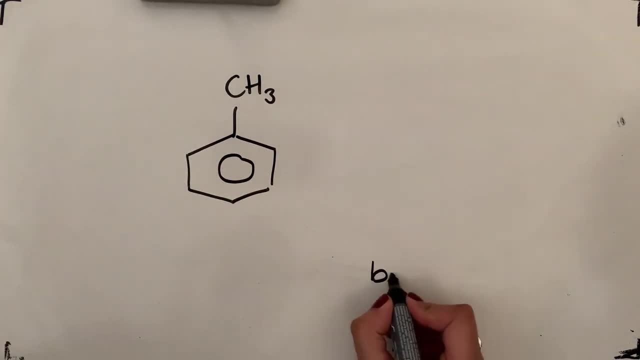 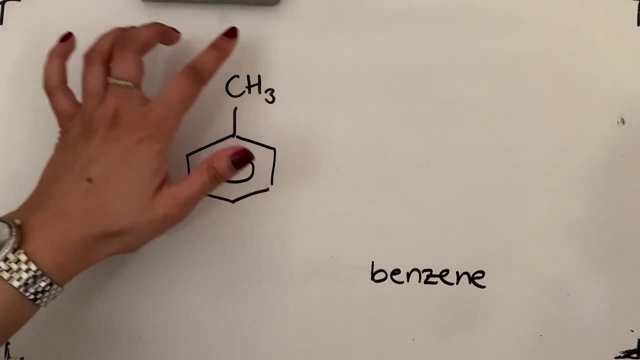 OK, so our benzene over here is our parent compound, So therefore the name is going to end in benzene And the substituent is anything coming off of that benzene. So we've got over here this alkyl chain. This one here is called methyl. 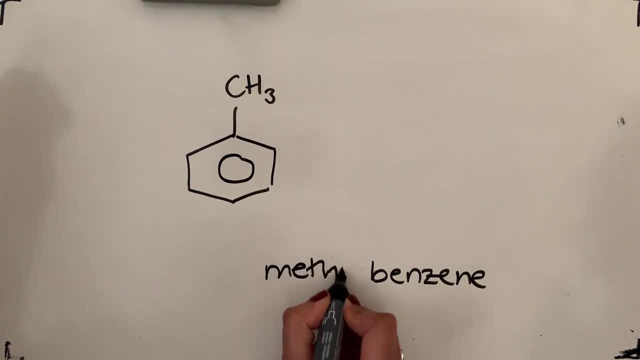 And therefore this compound here is just simply called methylbenzene. Right, Let's do another one. So if we've got this compound here, So again the parent is our benzene, So the name is going to end in benzene. 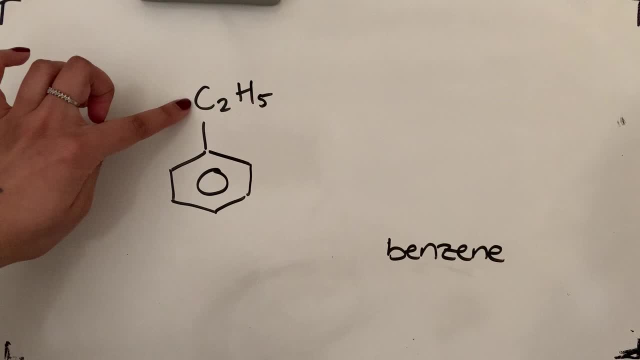 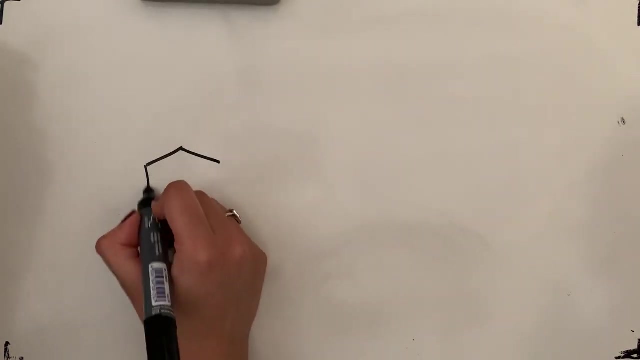 And now this alkyl group, here two carbons, and therefore this is ethyl. This compound here is called ethylbenzene, Fairly straightforward, Up until you get to seven carbons in the alkyl chain. So if you have to draw this out, one, two, three, four, five, six, seven, 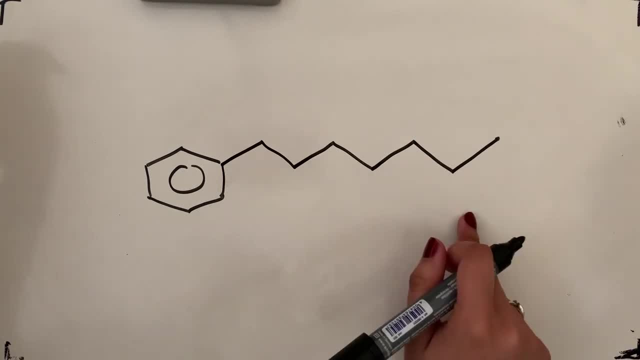 So, as you can see, we've got seven carbons in this chain coming off of here. If you have seven or more carbons in your alkyl chain, the benzene ring is no longer the parent compound. It becomes a substituent Right. 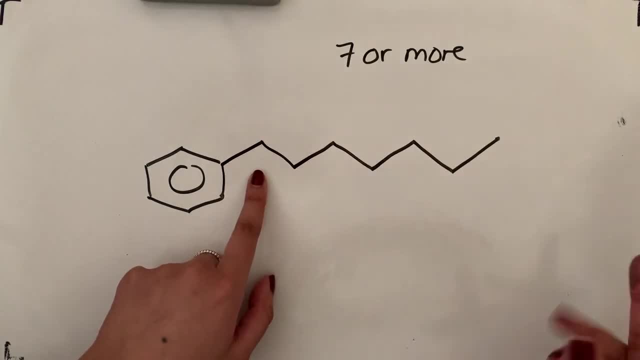 So now this alkyl chain is the parent compound. So let's just number this parent compound. So one, two, three, four, five, six, seven, You've got seven carbons and therefore it should end in heptane. 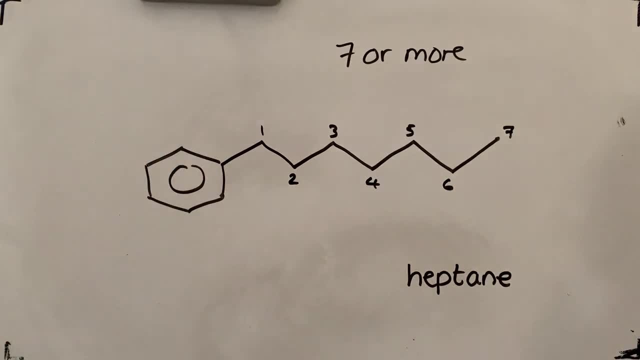 And now, as we said, this benzene ring is a substituent And as a substituent, we don't call it benzene anymore, We actually call it phenyl. So benzene rings as a substituent, We call it phenyl. 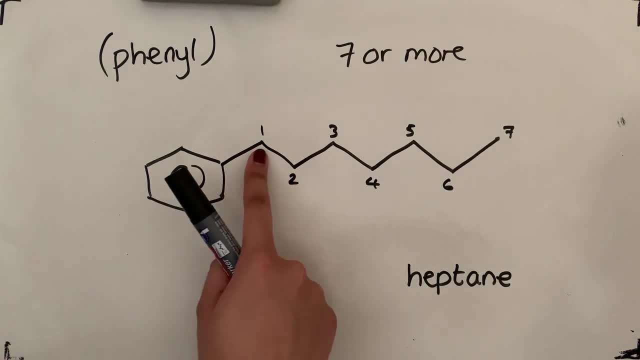 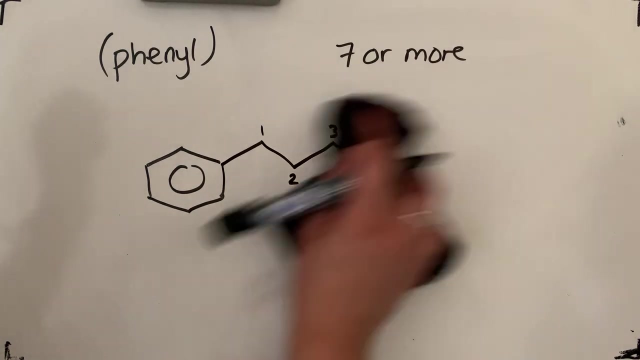 And, as you can see, this phenyl group is coming off of carbon number one, So this is called one phenyl heptane. All right, So if we have seven or more carbons coming off, benzene becomes a substituent. 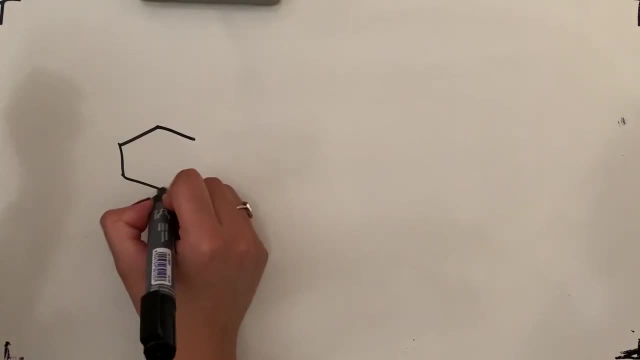 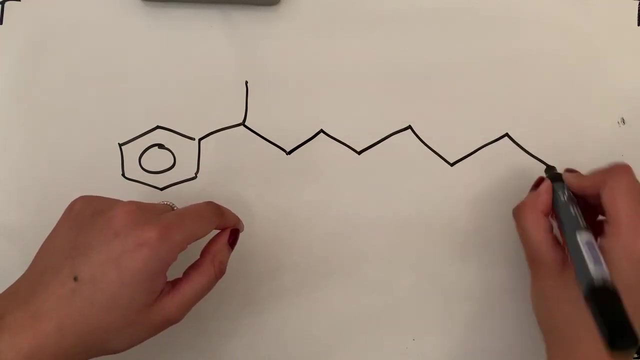 So let's just do another example of that. OK, so again we've got seven or more carbons coming off. In this case let's just see what the parent compound is. So I'm just going to number it one. So longest carbon chain actually starts from here. 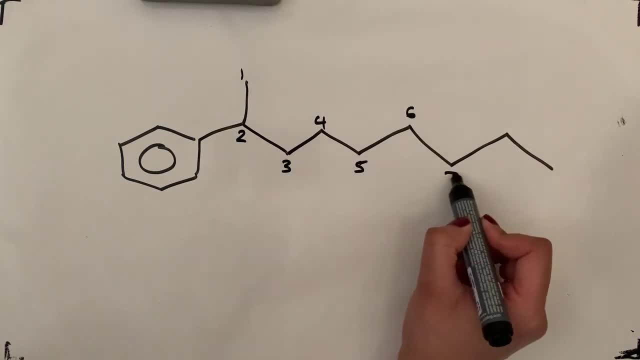 One, two, three, four, five, six, seven, eight, nine. So the parent compound is nonane, So it's going to end in the name nonane. We then look at the benzene ring as a substituent. 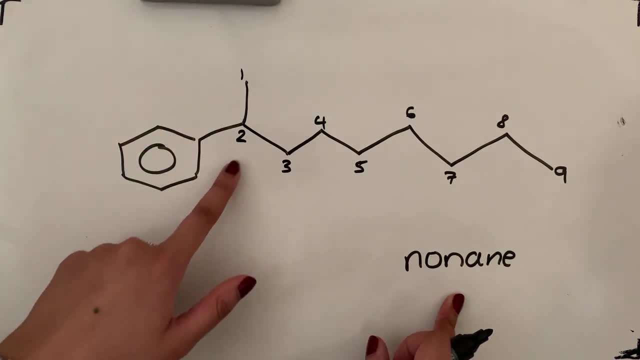 So again, it's going to be called phenyl. It's coming off of the second carbon, So this is called two phenyl nonane. OK, so the limit is up to six carbons. If it's got six carbons, it's going to be the benzene ring is going to be the parent. 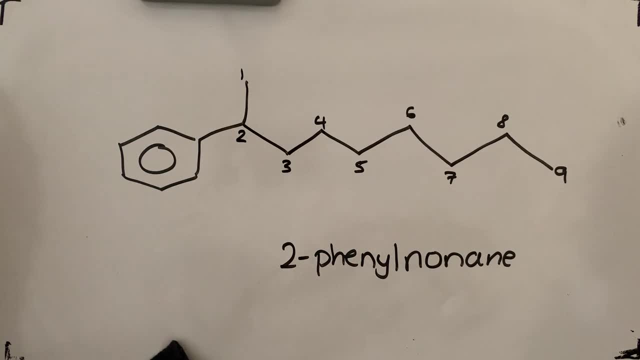 If it's got seven or more, it is going to be a substituent, Right, Let's look? Right, Let's look at compounds that aren't hydrocarbons. So let's say, in this one over here, we've got a chlorine atom coming off. 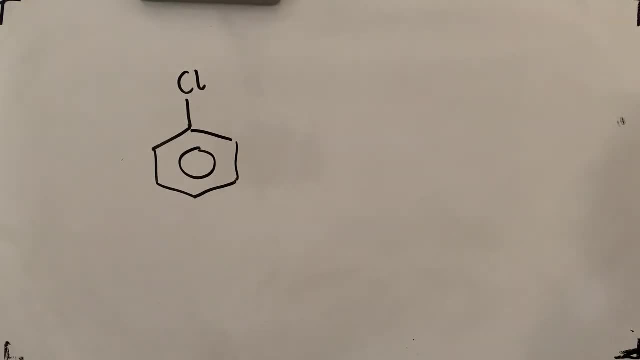 So again, your benzene ring is the parent, So it's going to end in benzene, and chlorine is as a substituent. It's classed as chloro, So this compound here is called chlorobenzene. Same applies for any other halogen coming off of it. 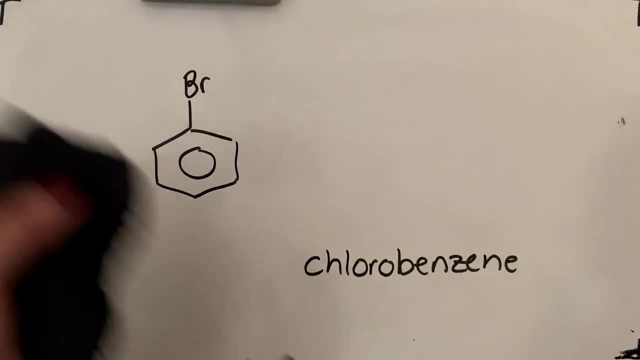 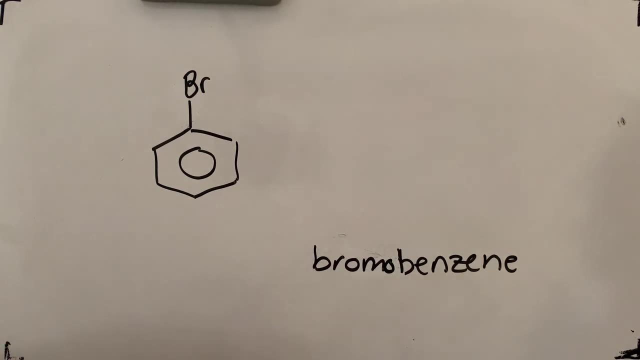 So, for example, if we had bromine, this would be called bromobenzene. If we had iodine coming off, it would be called iodobenzene. Thorine coming off, it would be called fluorobenzene, and so on. 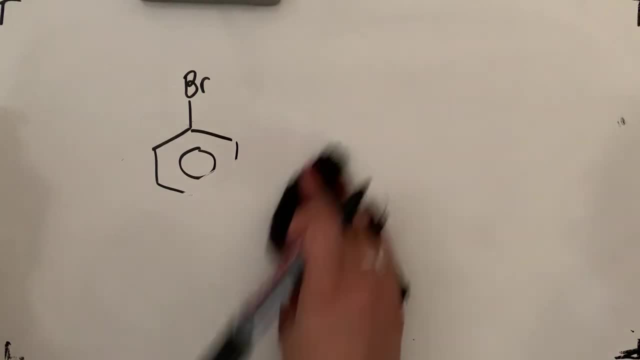 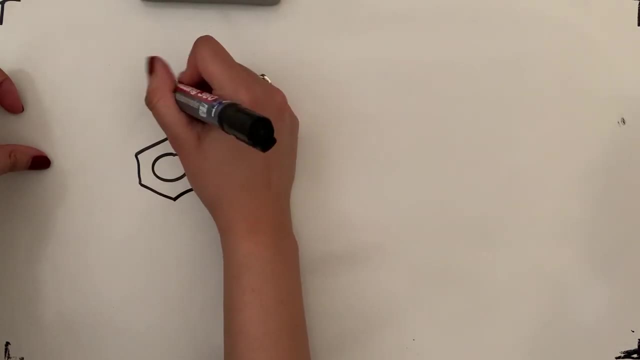 All right, OK, so that's the halogens and substituents done. Let's now just have a look at a new type of functional group that we haven't really covered, And that is this group over here. So we've got NO2, nitrogen based compound. 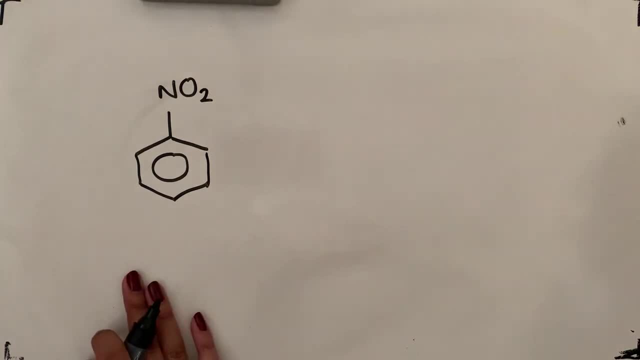 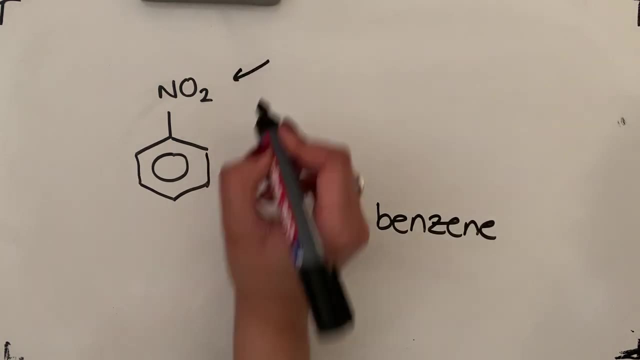 So let's have a think as to what this compound here is called. In this case, again, benzene is the parent, Now this NO2 up here we call this a nitro group, So therefore this compound here is called nitrobenzene. 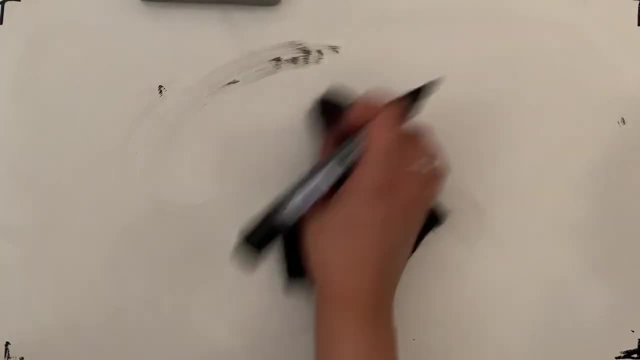 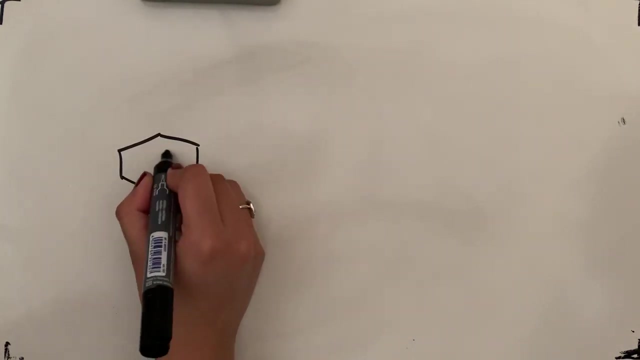 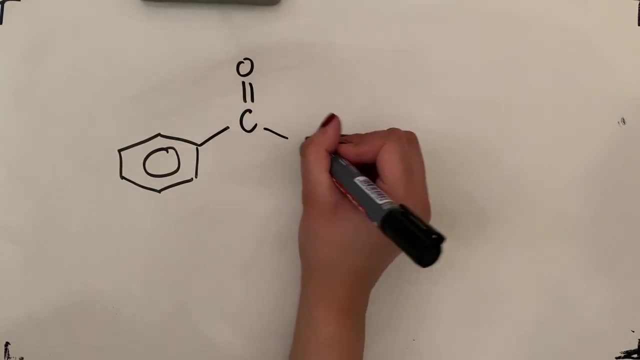 Right, Let's look at some more examples. So another one is where we have a carbonyl functional group coming off, So carbonyl being a C double bonded to an oxygen, So something like this. In this one, the functional group, we've got two functional groups. 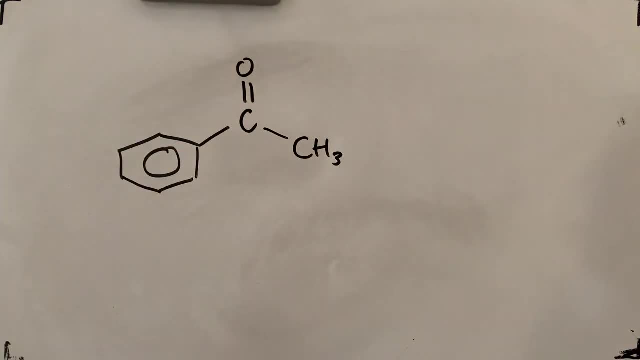 In fact we've got a carbonyl, so that's a ketone, And we've got a benzene ring, So we've got two functional groups. So we've now got to decide which one's the parent and which one is our substituent. 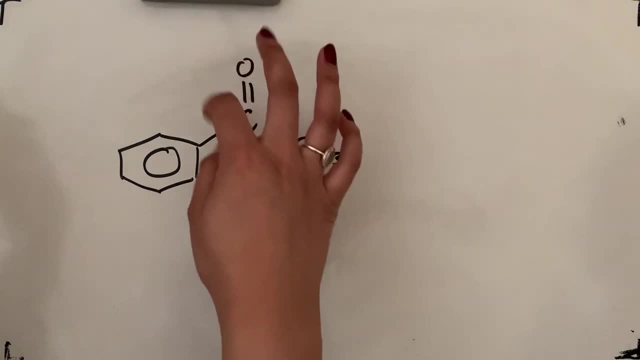 Now, in this case, when you have a ketone, a carbonyl, coming directly off of a benzene ring, this over here is going to be sorry. this whole thing over here is going to be the parent compound. So this one over here is a ketone. 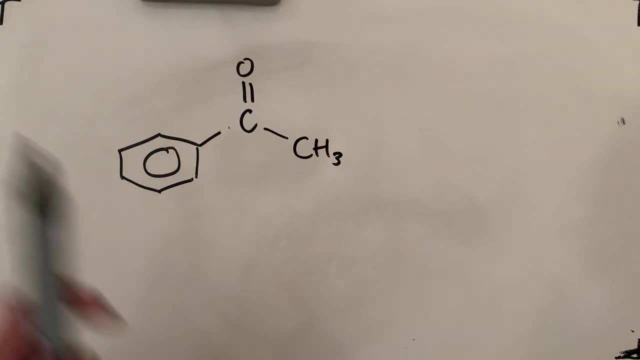 It should end in "-one". It's got two carbons And therefore this one is ethanone, So "-one" being a ketone, "-ether" being the fact it's got two carbons in it, So the carbon of the ketone is the parent compound. 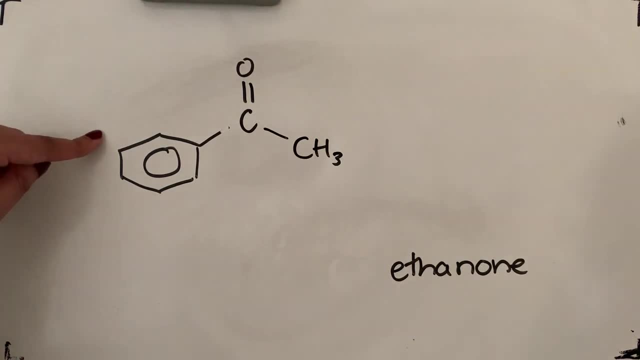 And the substituent is now our benzene ring. So as a substituent we call it phenyl And therefore this compound here is called phenyl ethanol. So that's the general rule. So that's the general rule. There are exceptions to these rules. 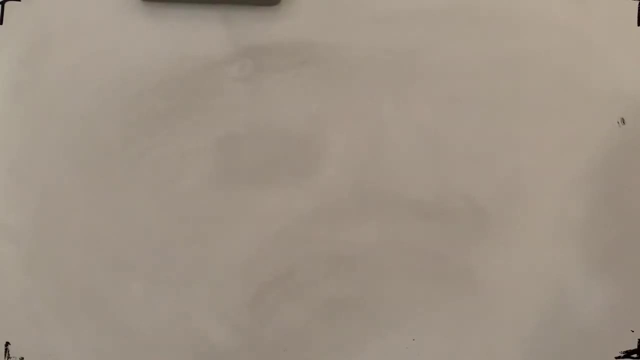 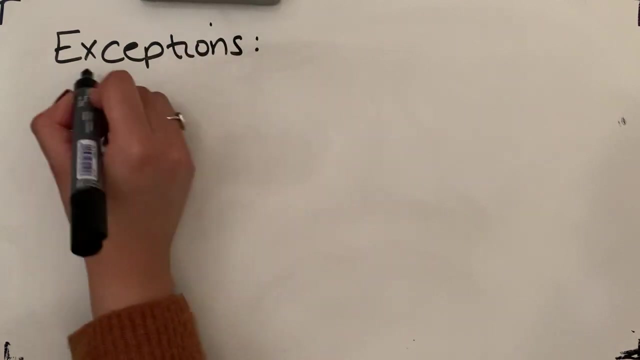 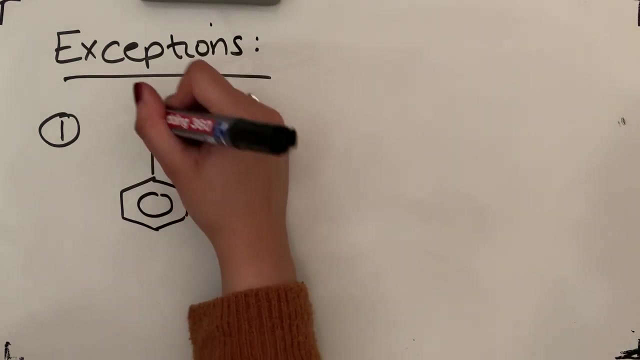 So the ones that you can't name, you just have to memorise the names. So the exceptions: there are three exceptions, So we're just going to have to memorise these names, The first one being this compound over here, Right, So, based on the rules that we've just covered, 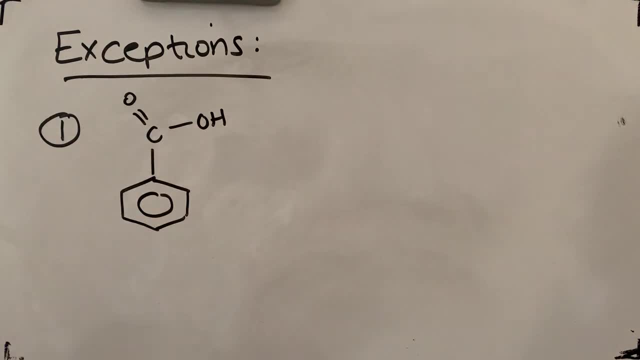 given that we've got a functional group coming off of our benzene ring, this should be the parent. It's a carboxylic acid. It's got one carbon, So therefore you would assume it's called methanoic acid. 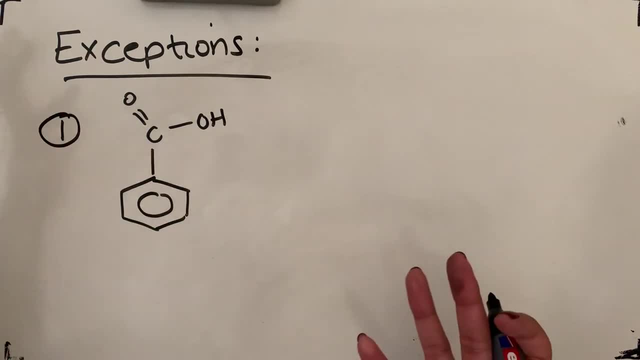 And therefore this should be a substituent. So you would assume it is phenyl methanoic acid. OK, The truth is, this is not the name. The name that we go for this one is benzene. It's a carboxylic acid. 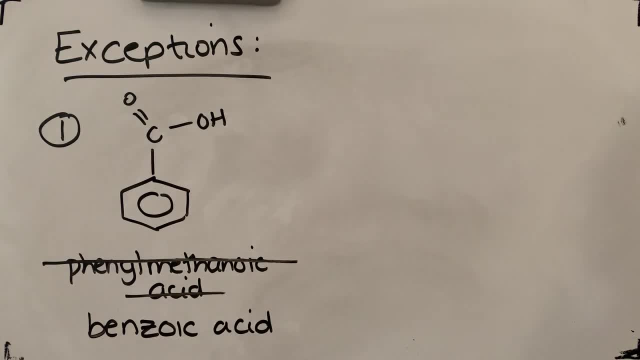 So it doesn't follow any of the rules that we've covered. This is one that you just have to know. it's an exception, Right? So that's exception number one. Don't know if I'm going to put them both on here. 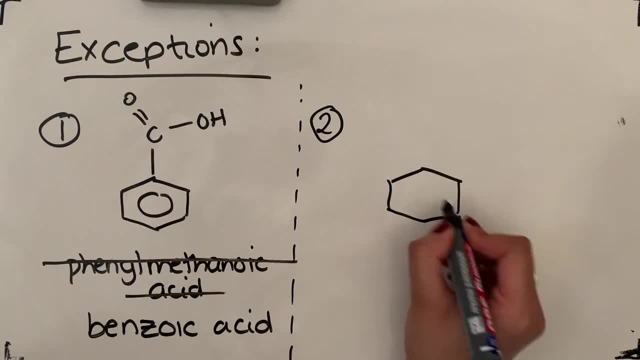 But exception number two is this one over here. So again I've got a functional group coming off the benzene ring. This one is an aldehyde, So it should end in al. It's got one carbon, So you'd assume it's going to end in methanal. 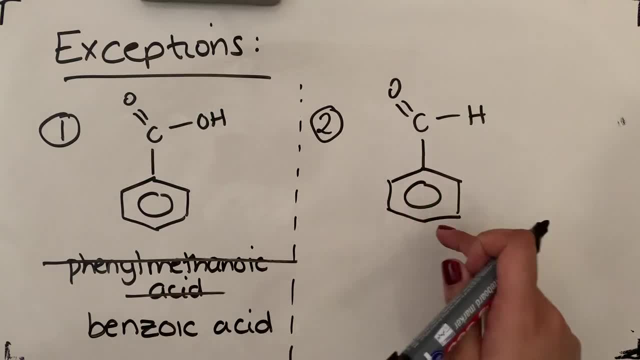 So, methanal being the parent compound, This being the substituent, So you would assume it is called phenyl methanal, Like that. Truth is it's not called that. We call this benzaldehyde, OK, so again a name you just need to memorize. 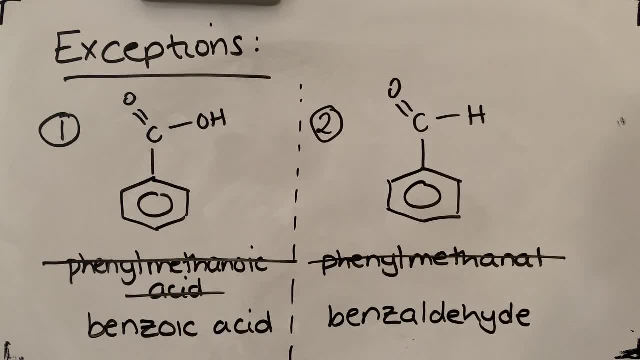 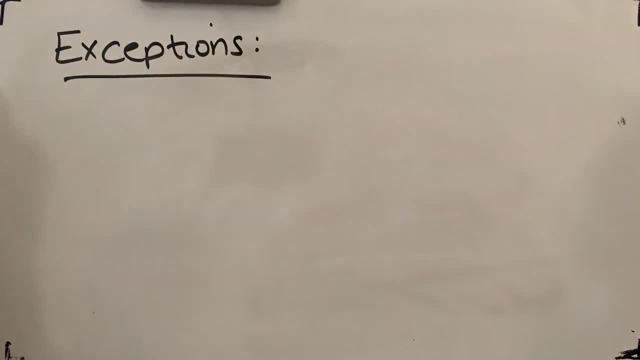 It's an exception to the rules that I've taught you. So that's exceptions one and two. I'm just going to cover exception number three. So exception number three is this one here. OK, so this over here is an amine group. 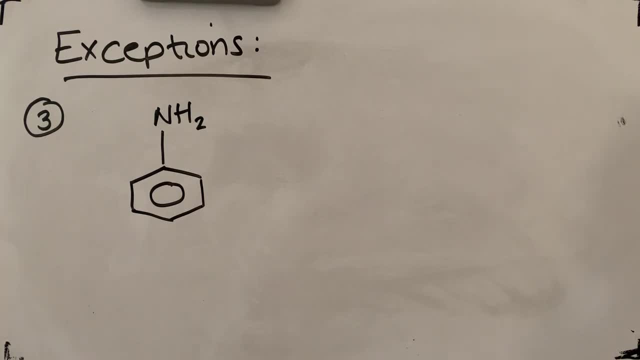 So usually when you're an amine group we give it the prefix amino And therefore you would assume this is called amino benzene. OK, don't worry too much if you haven't seen that amine group before. We do cover it later. 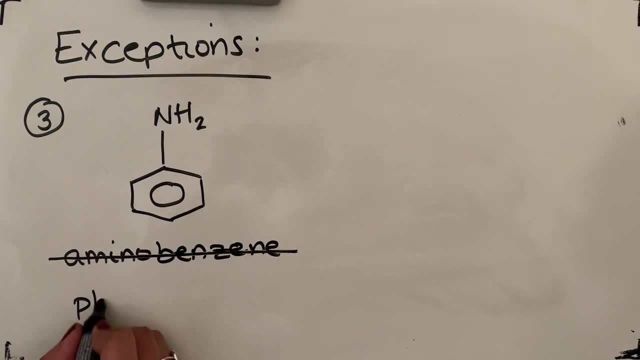 But the truth is it's not called amino benzene. We call this compound here phenylamine, Spelt phenyl amine. OK, so the amine in this case is actually the parent. The phenyl benzene ring is the substituent. 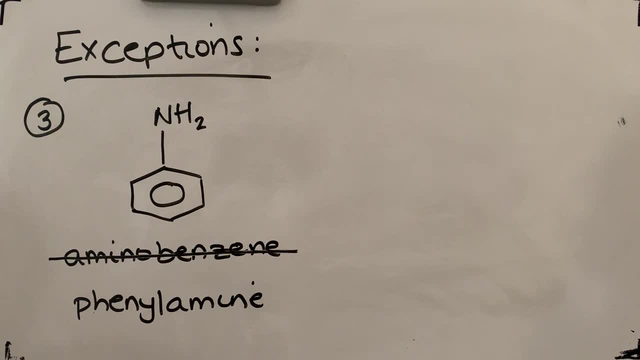 So this is called phenyl amine or pronounced phenylamine. So they are your three exceptions that you need to know. Let's now have a look at when you have more than one substituent on the benzene ring, Because so far we've looked at when we have just one substituent. 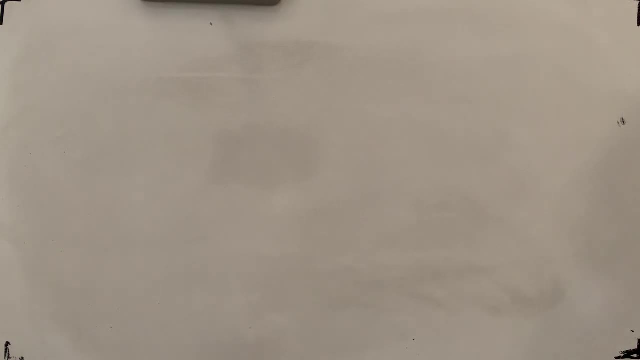 It's mono substituted. Let's now have a look is where we have di or more substituted benzene rings. OK, so first things first. The position of the substituents is now important, right? So what we're going to have to do is we number the carbon atoms in our benzene ring. 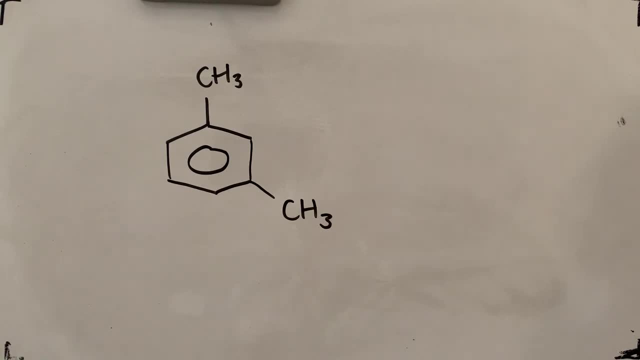 So that's important. It'll tell us which number carbon we find those substituents on Right. So again in this one we've got a benzene ring That's going to be our parent. We've got our methyl groups. 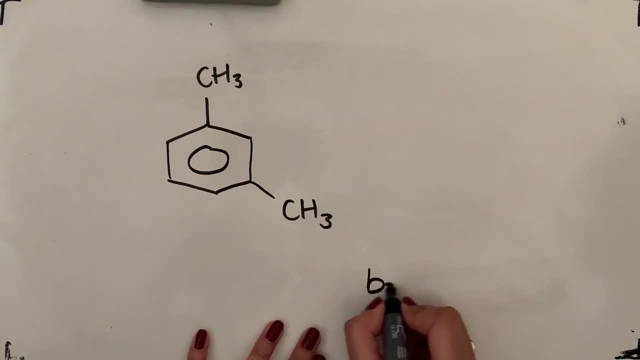 They are substituents, So it's going to end in benzene. It ends with a parent name. We now have two methyl groups, So two methyl groups. So therefore we call it dimethyl. So we've got dimethyl benzene. 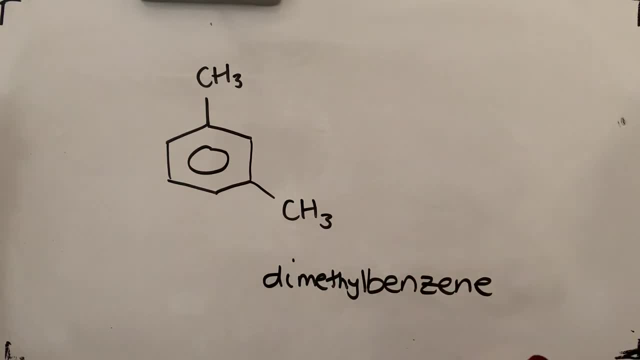 But those methyl groups at the moment could be on any carbon, So we now need to specify which carbon they are found on. So the aim is to have the methyl groups on the smallest number carbon. So the best way to do that is start as that one being number one. 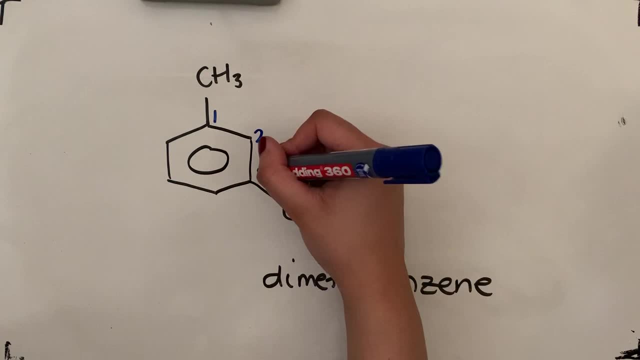 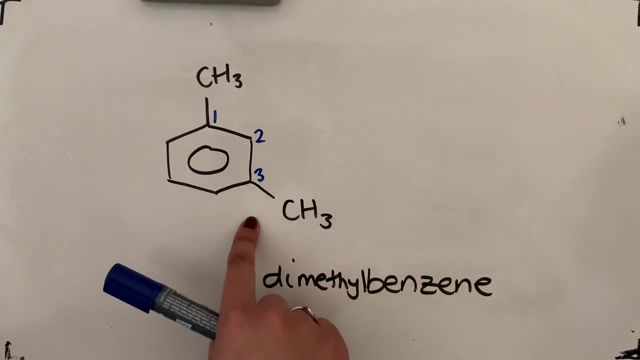 If I go clockwise, this one will end up on number three. I don't want to go anti-clockwise because that's going to therefore end up on one, two, three, four, five, And that's a bigger number than three. So this compound here is therefore called 1,3-dimethylbenzene. Right, Let's move on. Let's try This one here. So again, we've got a parent compound. This one is benzene, And we've got three chlorines attached to this one. 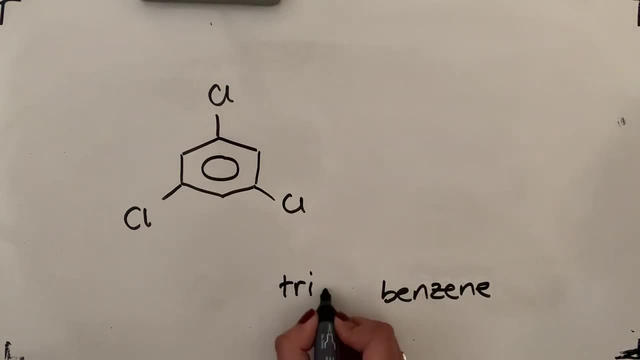 So this is going to be trichlorobenzene, Trichlorobenzene, And again you've got to put numbers on your carbons in the benzene ring. In this one, it doesn't actually matter which direction you go in. 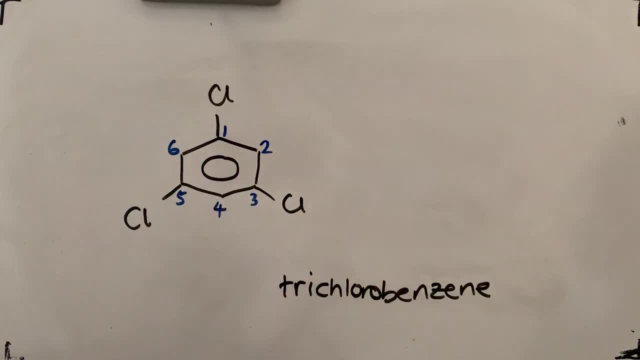 So, as you can see, this is called one, Three, Five. So you put those numbers in order. It's one, Three, Five, Trichlorobenzene. OK, let's do another example where we now have different types of substituents. 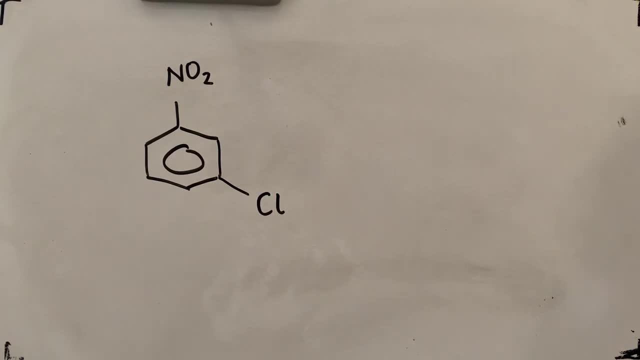 Like so. So what we now need to do is decide how to know This one. Now again, we've got a nitro compound. We've got a chloro. That's where we got nitro Substitution. We've got chloro substituent. 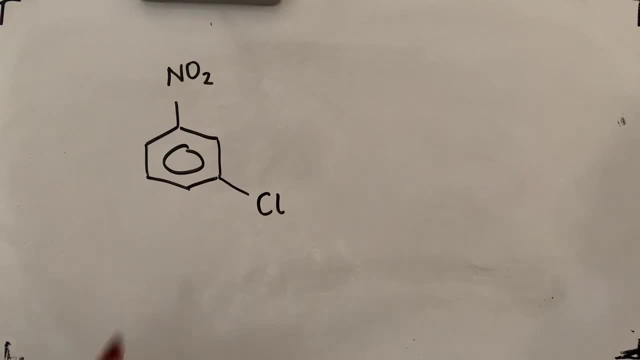 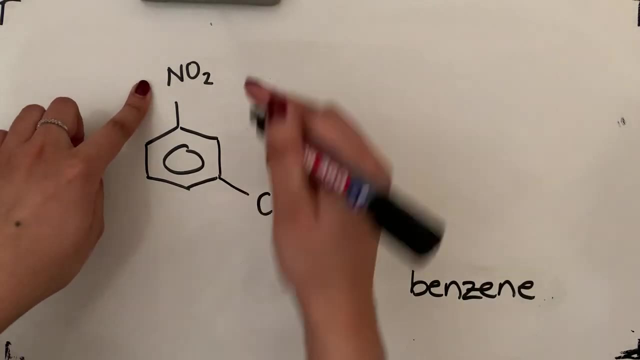 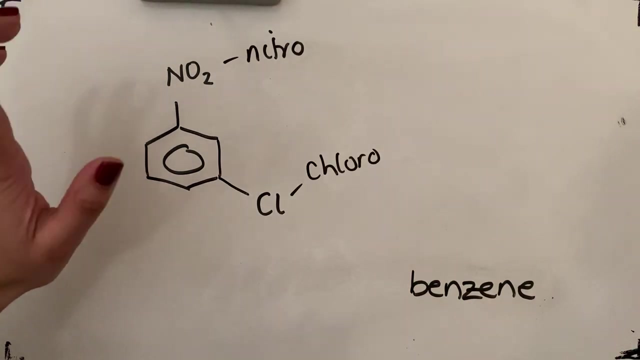 In this case, your benzene ring is the parent, So the name is going to end in benzene. We've got two substituents: We've got nitro And we've got chloro. OK, What you now need to do is put them in alphabetical order. 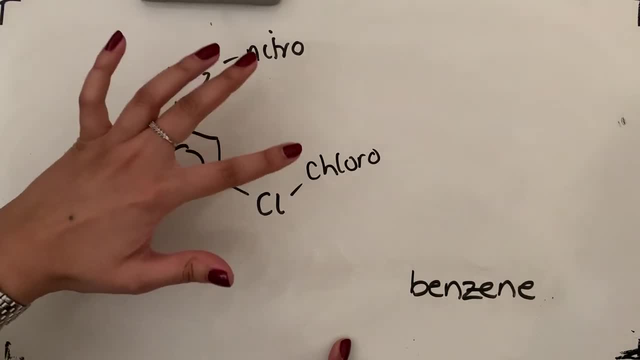 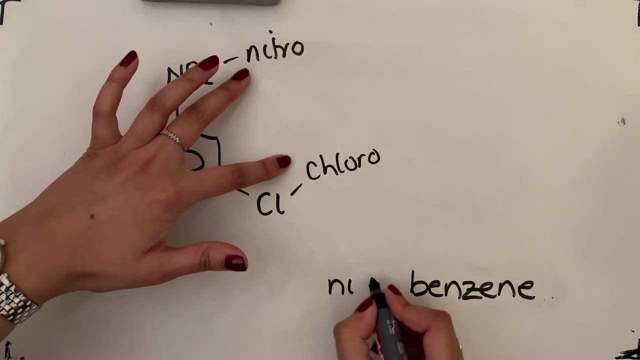 So chloro goes before Chloro goes before nitro. You pick the one that is last in the alphabet, So in that case it's going to be nitro And you put that with the benzene, Like so, And the one that is last, the one that you've put with benzene. 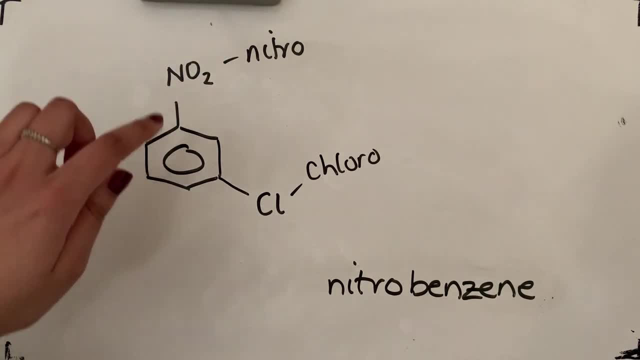 the carbon to which that is attached to becomes carbon number one. So this has got to be carbon number one, And then all you do is you number to put. So I'm going to go clockwise to put the chloro. It's on the smallest number carbon. 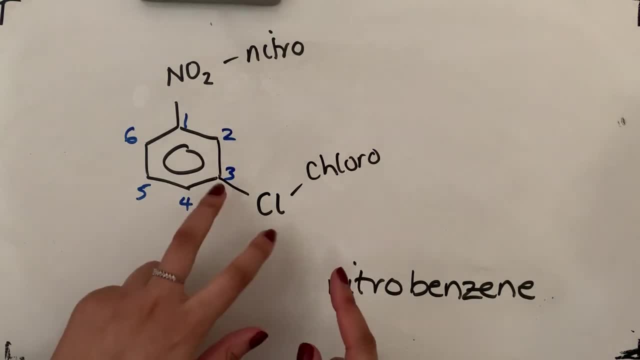 And now you put the first. So the first one in the alphabet was chloro. You give that the number three. So therefore this compound here is called three, chloro nitro benzene. You do not need to put the one with the nitro. 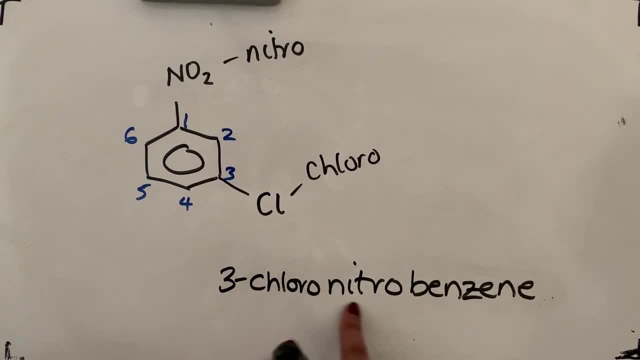 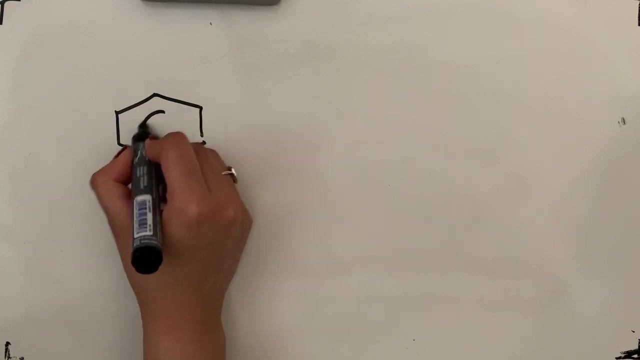 because putting nitro with benzene tells you that that nitro is already on carbon number one, So you don't need to call this three chloro one, nitro, benzene. So that's another example, Right? So two substituents. 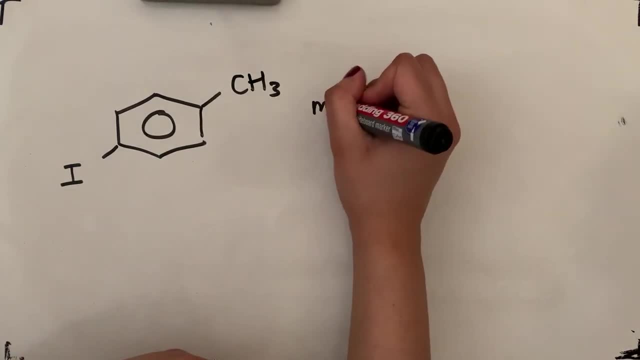 Again, we've got iodo. We've got methyl to write them down. So you've got methyl and you've got iodo. So again, the parent compound here is benzene. It's going to end in benzene. You now decide, out of iodo and methyl, which one is last in the alphabet. 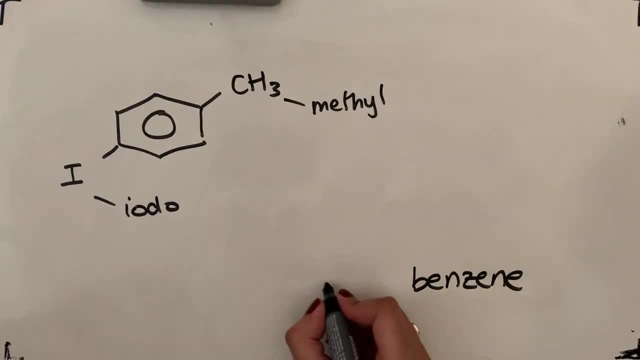 In this case it is methyl. So you put methyl with benzene and your methyl, the carbon to which the methyl is attached to, becomes carbon number one Again. it doesn't matter which way I number now, And therefore your iodo is on carbon number four. 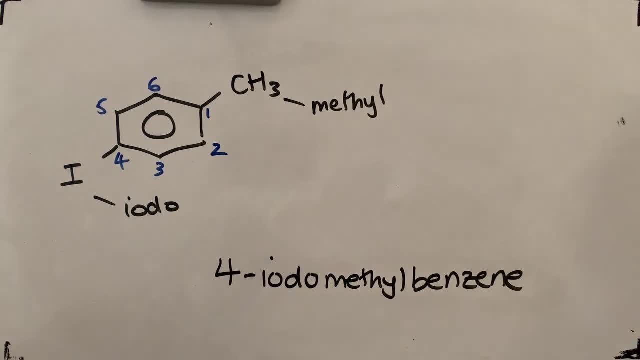 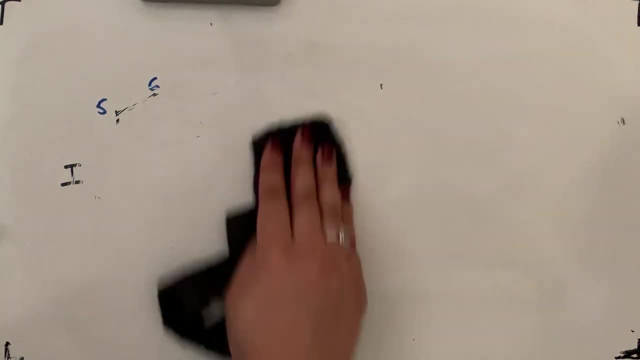 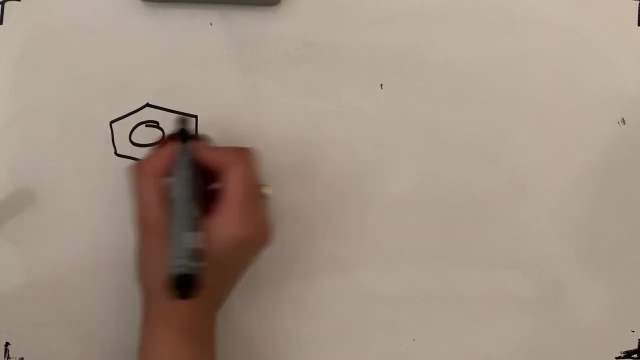 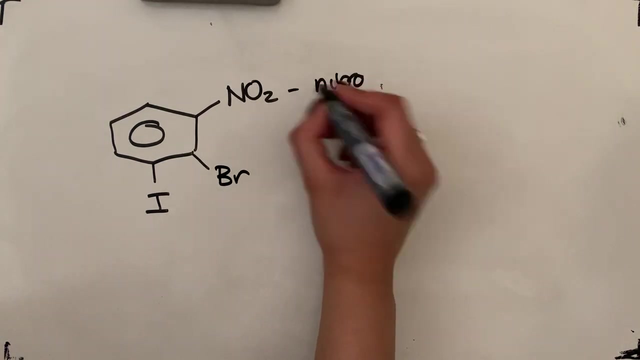 So, therefore, this is called four: iodo methyl benzene. Let's now have a look when we have three substituents. So we've got in this one, we've got nitro, We've got bromo And we've got iodo. 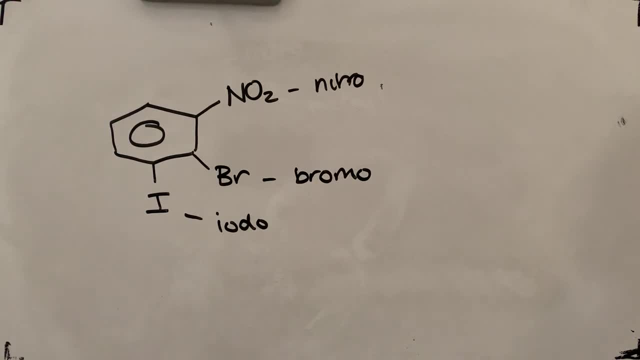 Right. So again in this case, the parent compound is our benzene. Again, out of all three of these, which one is last in the alphabet? In this case it's our nitro. So nitro goes with benzene and our carbon with the nitro. 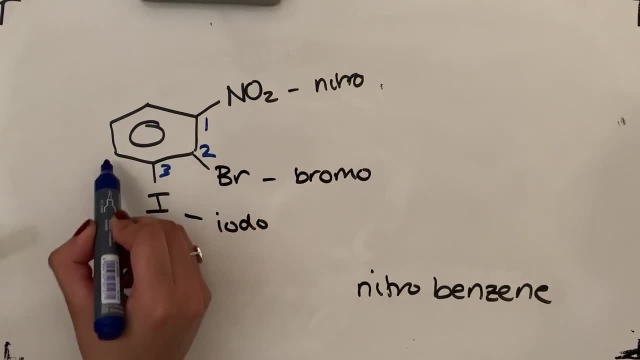 Becomes number one. Keep going in this direction. And now we've got to put our bromo and our iodo in order. You again go alphabetically. So first in the alphabet, and therefore first in the name, should be your bromo. 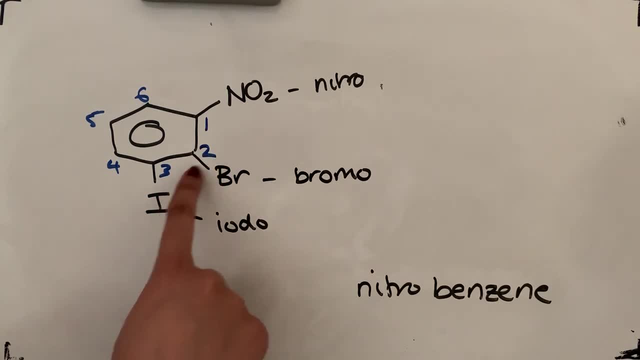 Doesn't matter about the number it's attached to. You don't go in the order of the numbers. You go in the order of the alphabetical names, and therefore bromo is first. So it should be. So. bromo is, on carbon, number two. 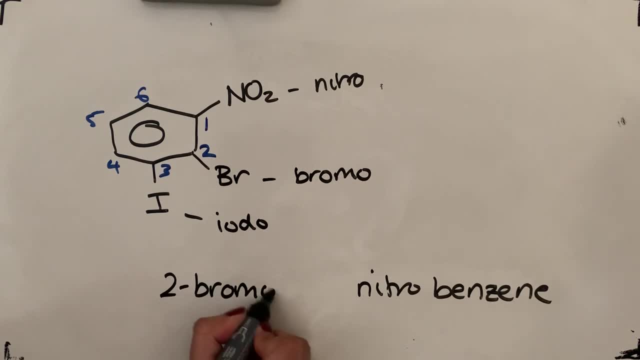 So it should start off with two bromo, And then we have three: iodo, Nitro, benzene. So just bear in mind, These three are in alphabetical order always, And the one that is last is technically is classed as your carbon number one. 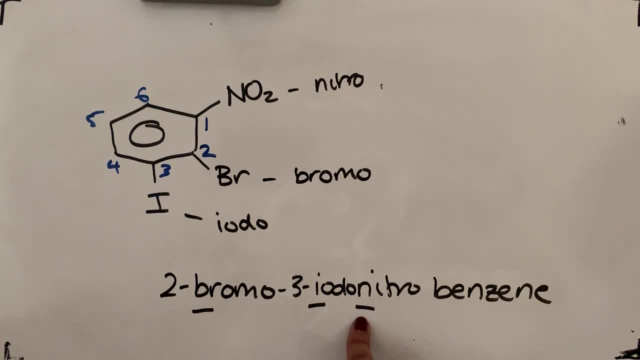 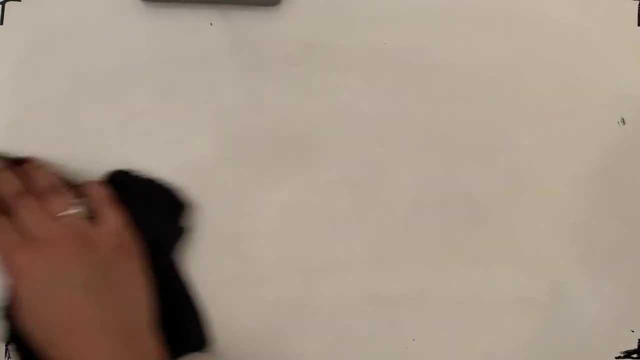 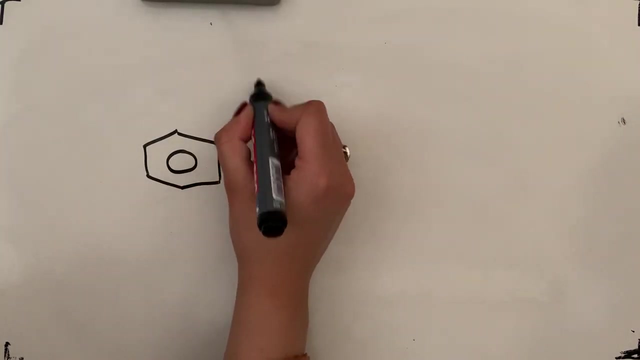 You don't need to put the one in front of in this one In this case, Don't need to put the one in front of nitro Right Last example. So we've got two substituents coming off here, But now remember, the benzene ring is not the parent compound. 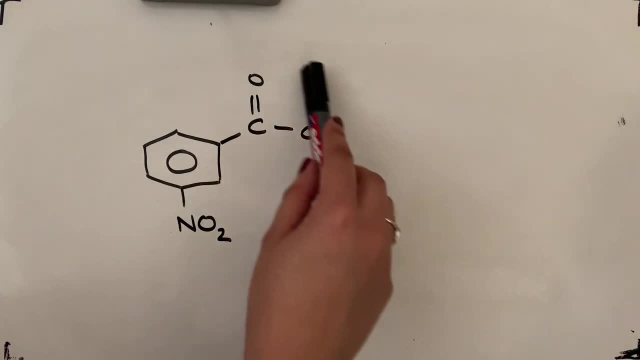 Because This compound here is one of your exceptions. So always remember, always look for those exceptions because they are more important And therefore they are the parent compound. So in this case, This compound here is your parent compound, If you remember, as we've covered, it is called benzoic acid. 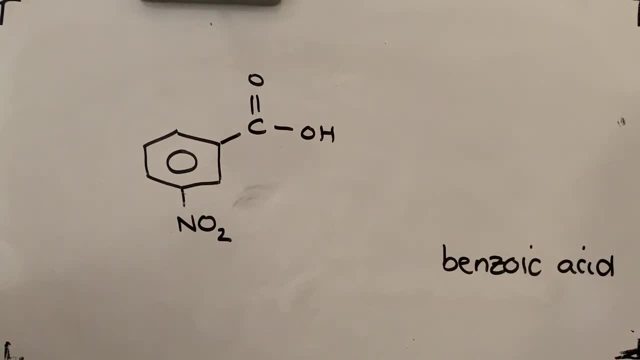 So therefore this is going to end in benzoic acid And the benzoic acid, So where the acid part is coming off, That is carbon number one Always, And therefore this compound here Is called Three Nitro.